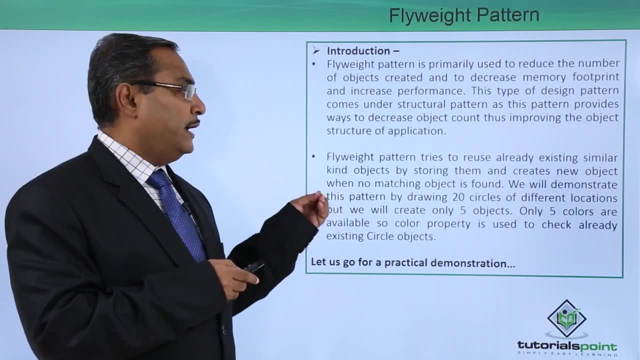 tries to reuse already existing similar kind of objects by storing them and creates new object when they are not in use. In case of flyweight design pattern, we shall always try to optimize the number of objects which are getting created so that we can have the lesser amount of memory. 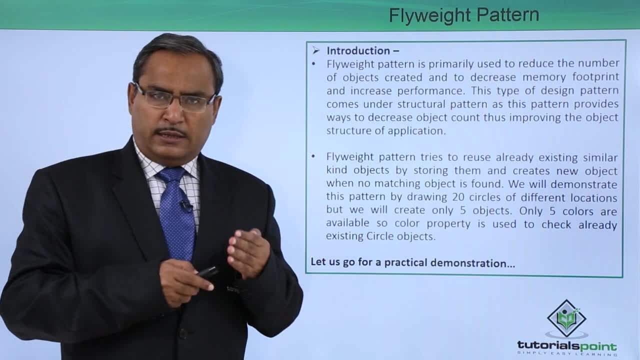 during the runtime of the system and also to increase the performance of the system and also to increase the performance of the system and also to increase the performance of the system when no matching object is found. So whenever some pre-existing object can come in our purpose, then we will. 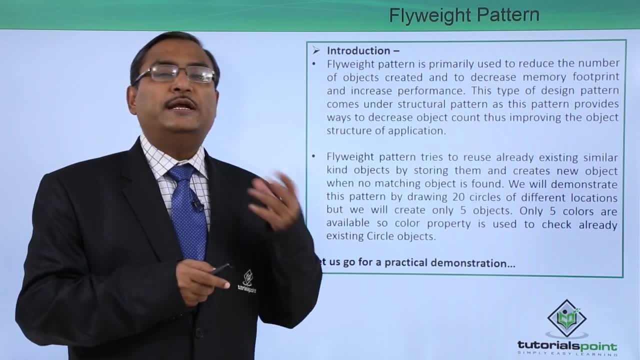 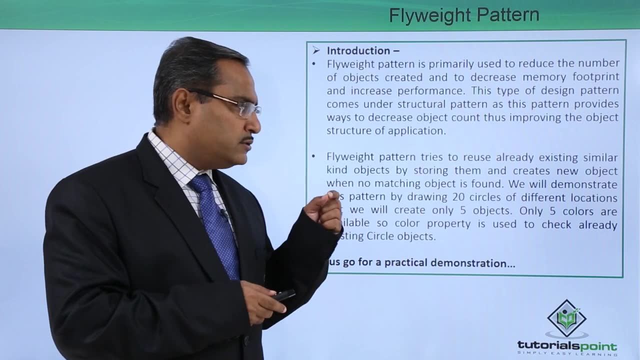 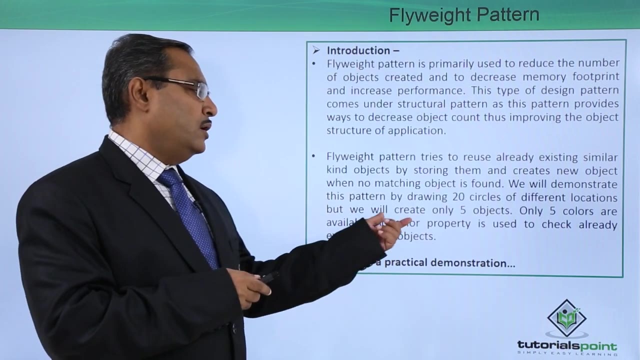 be reusing the pre-existing object, but if the object is not pre-existing, then only the new objects will be created. We will demonstrate this pattern by drawing 20 circles of different locations, but we will create only 5 objects. Only 5 colors are available, so color property. 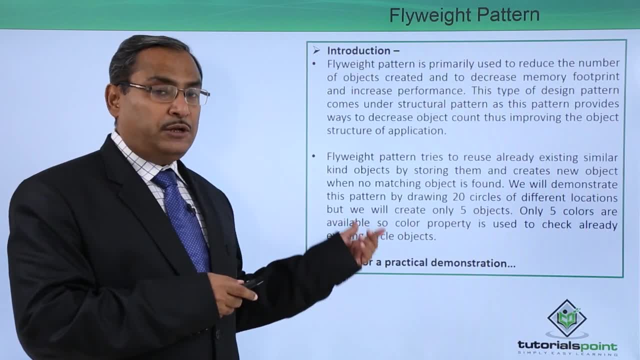 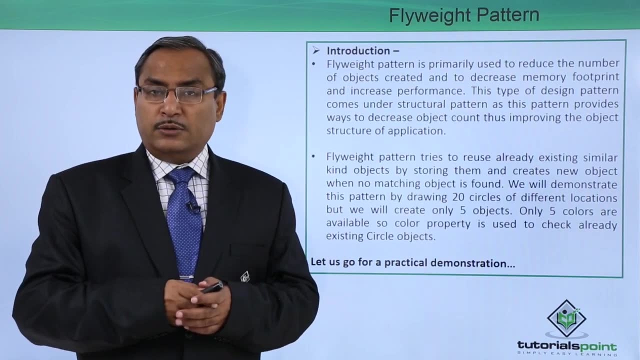 is used to check whether the object of the object is available or not. In case of flyweight design pattern, the object of this particular circle is pre-existing or not. So let us go for one practical example, and there we will be showing you one Java application and also we shall explain our case. 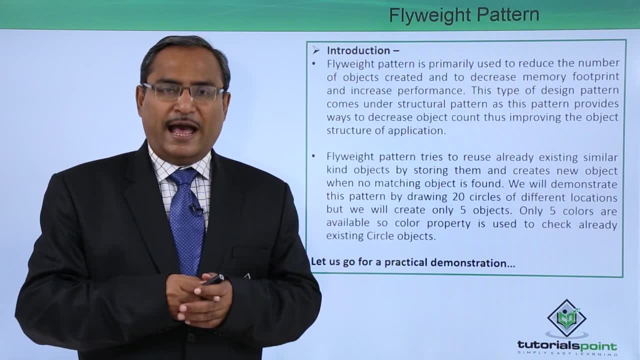 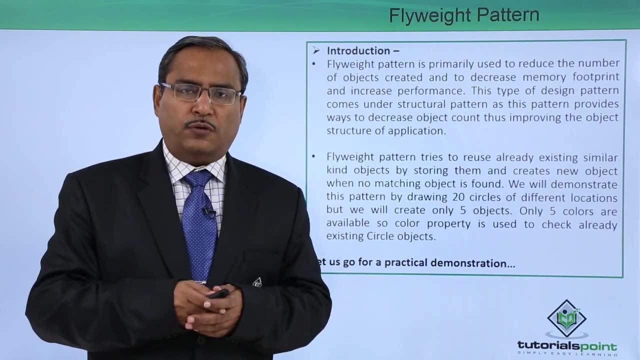 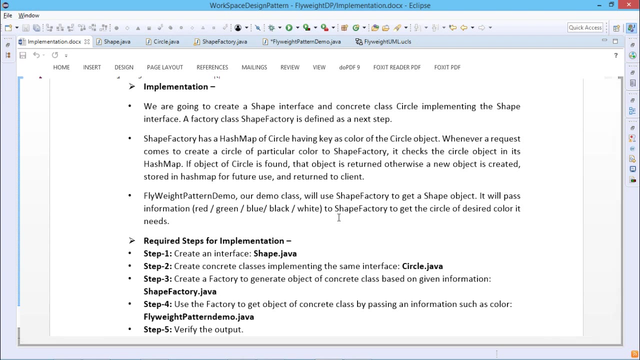 study with UML class diagrams and for the better understanding, this demonstration will help you to learn about this concept. So here is the demonstration for you. Flyweight design pattern is one of the structural design pattern, as this pattern provides ways to decrease the object count, thus improving the application required: objects, structure and 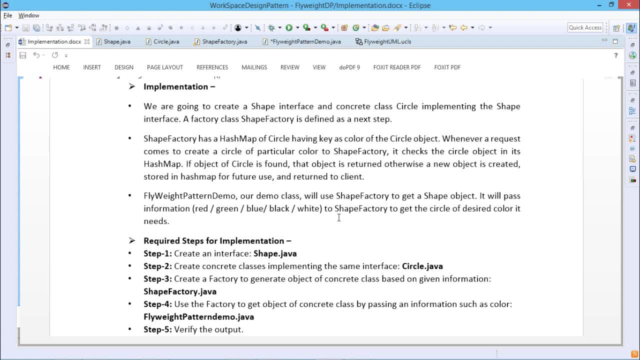 flyweight pattern is used when we need it need to create a large number of, a huge number of similar types of objects. let let it be say 10 to the power of 4 or 10 to the power of 5. number of, and one important feature of flyweight objects is that they are immutable. That means they cannot be modified. 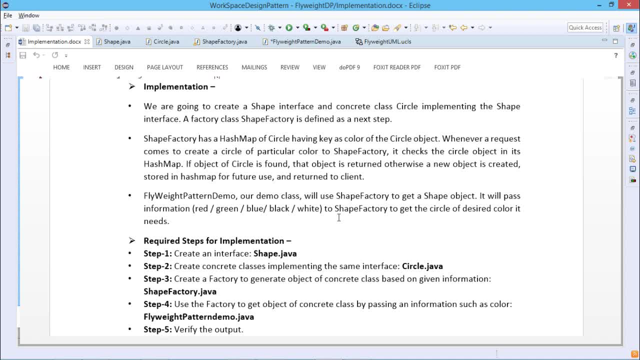 once they have been constructed. So now let us go to have one implementation of this flyweight design pattern using our Java coding. and we know that whenever we are having the lesser number of objects which will reduce the memory usage, and it manages to keep us away from errors related to the memory, like the error message that 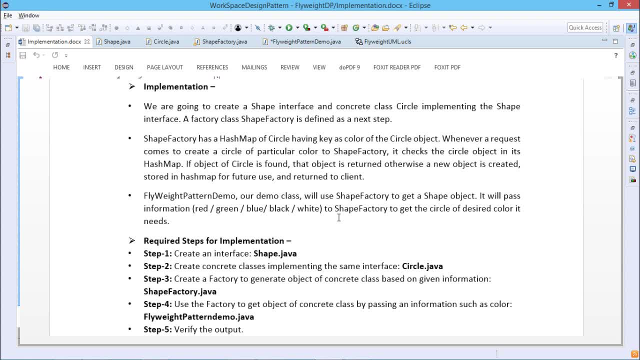 is the javalangout of memory error and although creating an object in error, java is really fast and you can still reduce the execution time of our program by sharing our object. so here we are going to create one shape interface and concrete class circle implementing the shape interface. the factory class, that is, the shape factory, is defined as a as. 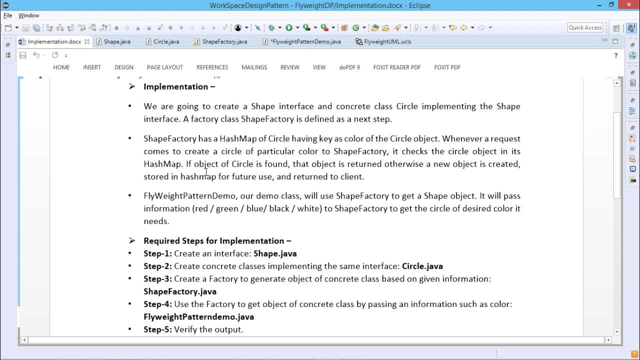 a next step and shape factory has a hash map of circle where the key will be the color and the circle object will be the value. so whenever a request comes to create a circle of the particular color to the shape factory, it checks whether the circle object is there in the hash map. 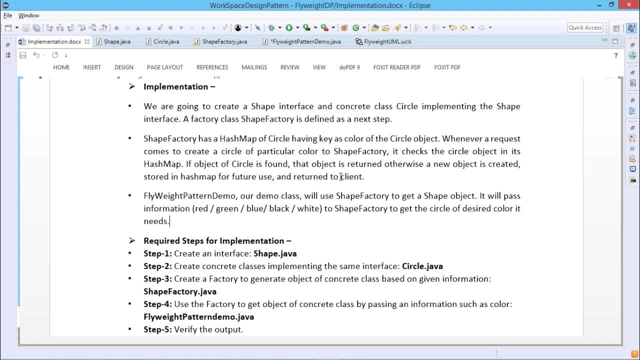 or not. if the object of the circle is found, then the object is returned. otherwise a new object will be created, stored in the hash map for the feature use and returned to the client. flyweight pattern demo will be about demo class and will use the shape factory to get a shape object and it will 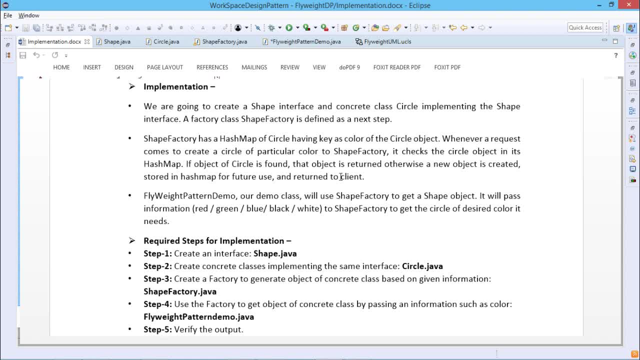 pass the information. let it be green, or say red, green, blue, black and white to shape factory, to get the circle of the desired color as it needs. so now let us go to implementation. go for the implementation step by step. so at first we are going to create one interface, that is the shapejava. so this is our shapejava. you can find that public. 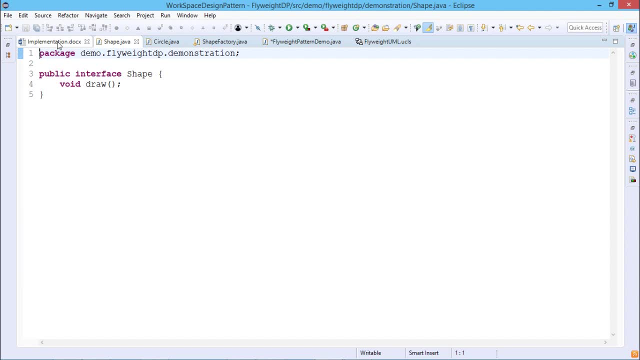 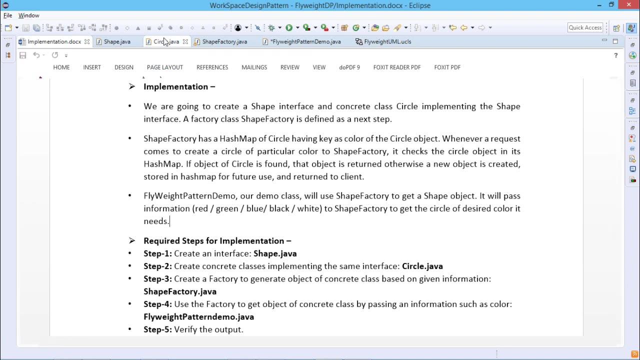 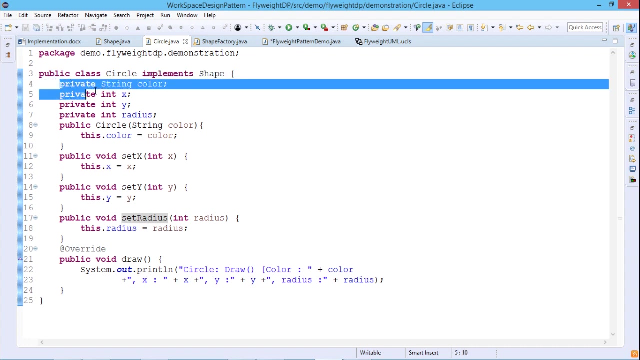 interface shape and it is having only one method, that is, draw. next, we are going for one concrete class implementing a shape interface. that is my circlejava. so let us discuss this circlejava, which is implementing the interface shape, which is having the instance variables. all of them are: 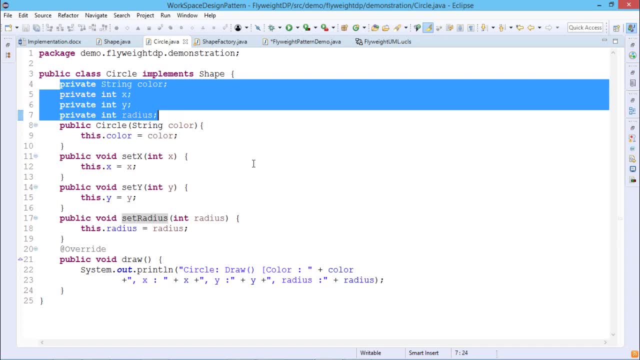 the private scope, that is, the string color, int x, int y and int radius and circle, is nothing but a constructor. so, according to the input parameter which will be passed, that is, the parameterized constructor, this color will be instantiated accordingly, will be initialized accordingly. we're having this public void set x, which will, which is the setter function for the. 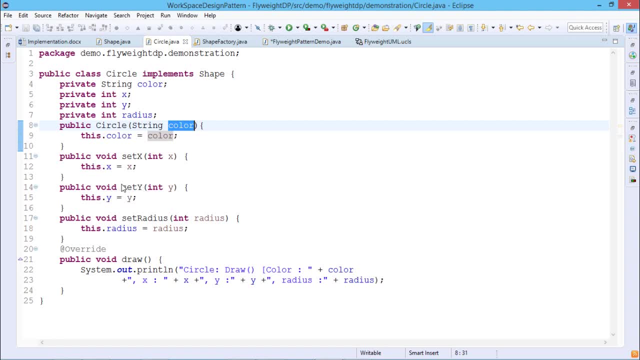 int x. this is a setter function for the y, so the name of the function is method is our setter function for the y, so the name of the function is method is our setter function for the. if we are execute in the執方, let's go ど. 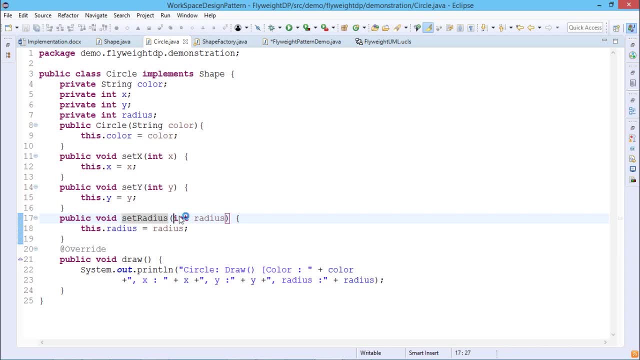 Y, and here we're having this set radius, which is taking this radius as input parameter and instantiating this particular radius, That is the instance variable radius. and here we are having this draw which will print the color, which will print the X, Y and the Radius values. So we are, we are having this circle dot Java. Let us go for this shape: factory dot Java. 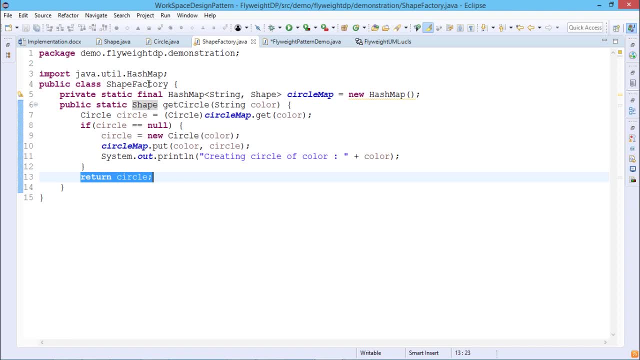 Let us go for this shape factory dot Java. So public class shape factory. So there is a class we are going to define and private, static, final hash map. So you know that hash map. in this case we are having a key value pair. So key is the color, which is B, which will be of the type string and value will be the shape class object. 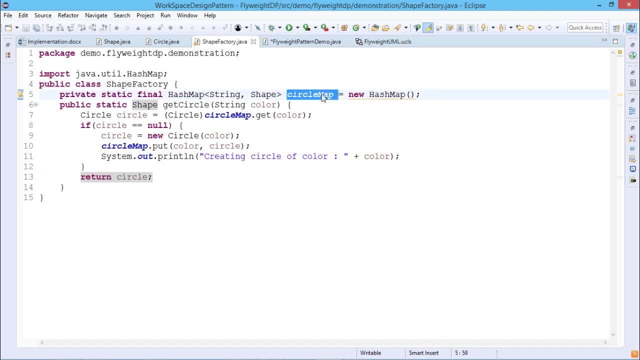 This hash map object name is circle map and it has got instantiated. We're having one method that is a great circle. This get circle is taking this color as input argument, as input parameter, and it returns the shape object and As output. so circle circle is equal to circle. 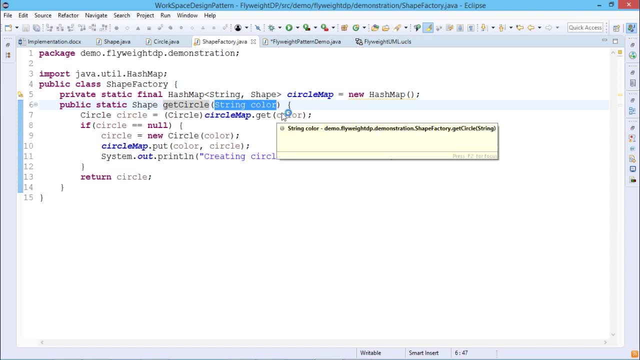 Circle map dot get color. So depending upon the color treating it, treating it as a, as a key value. So circle map is actually returning the circle class object, But if the color does not match, then the circle object will be having the value null. if the color is matching, then obviously, 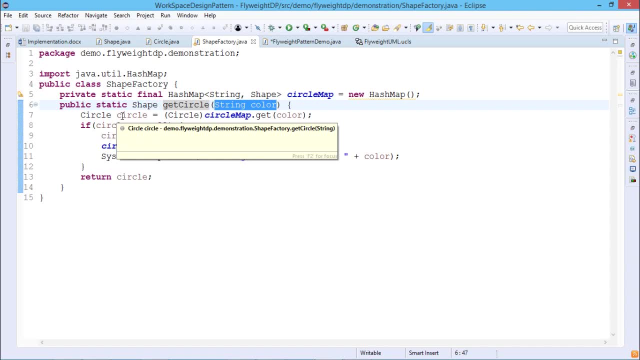 Circle will be having the respective object retrieved from the hash map circle map. So here we are having this: if the circle is equal, is equal to null, Then we are going to create a new circle object and we are putting this color there. We are putting this color as through the constructor and then with this color value, 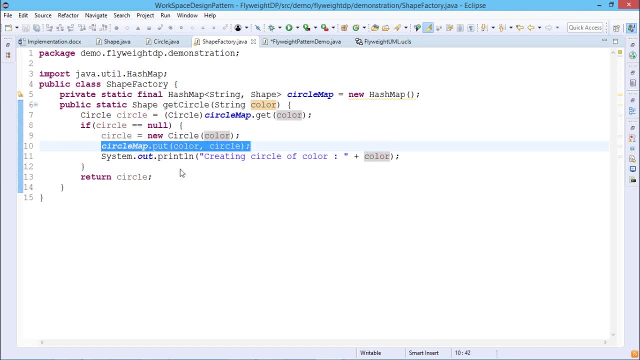 We are putting it into the circle map hash map. So using the method put, and here also we are printing one line, That is the one string will get printed. that means the new circle has got created with this color and then either the Retrieved circle object from the circle map hash map, that will be returned. 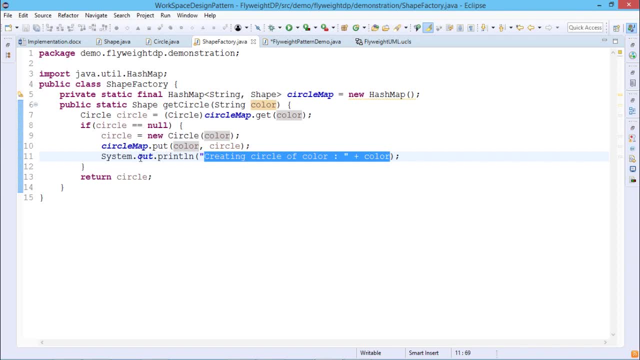 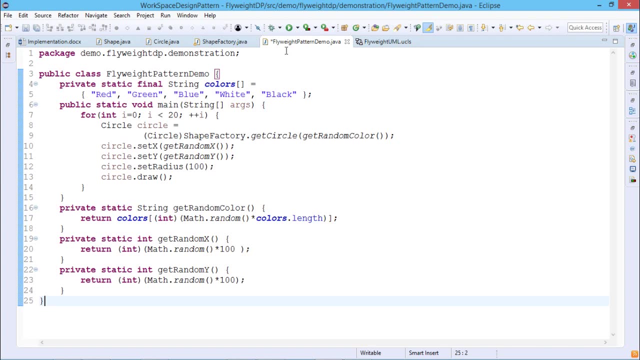 Or if the circle is equal to null, then the new circle, whatever has been the object We are going to create, and that will be returned at the end. Next we are going for this fly wet pattern demo. So now we have finished up to the step number three. 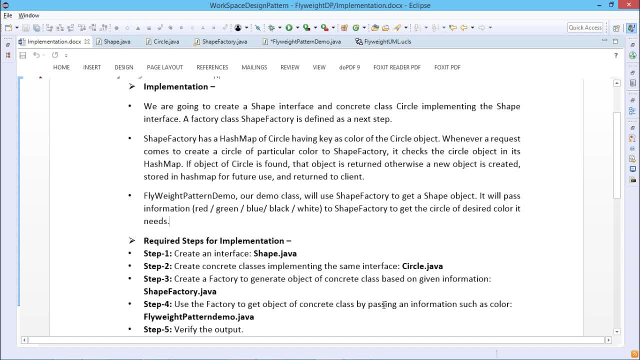 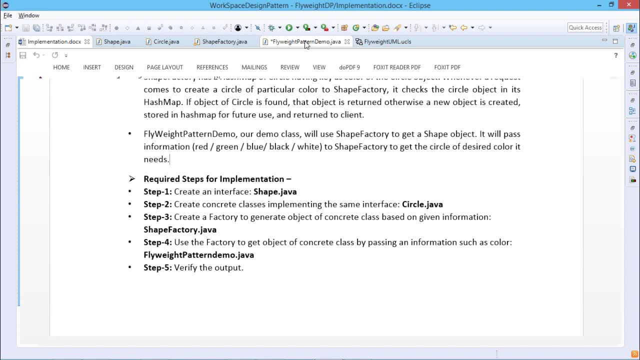 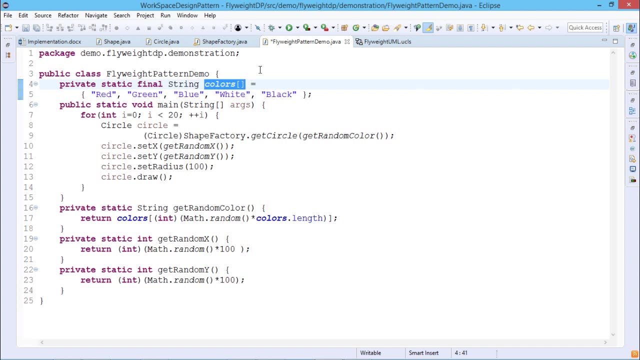 so use the factory to get the object of concrete class by passing an information as such as a color, and Fly wet pattern demo dot Java is the respective class name. So here we are having this fly wet pattern demo dot Java, Under which we are going to define one final array, static final array, which is containing string type of objects. 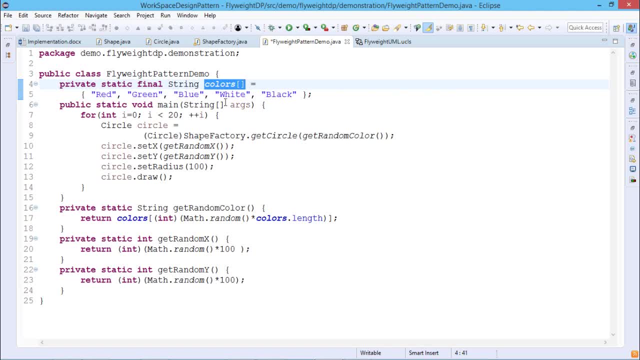 So that is a red, green, blue, white and black. So the size of this array is 5. So now what we are doing is the main function we are having. so one for loop is executing from 0 to 19, so circle circle is equal to. 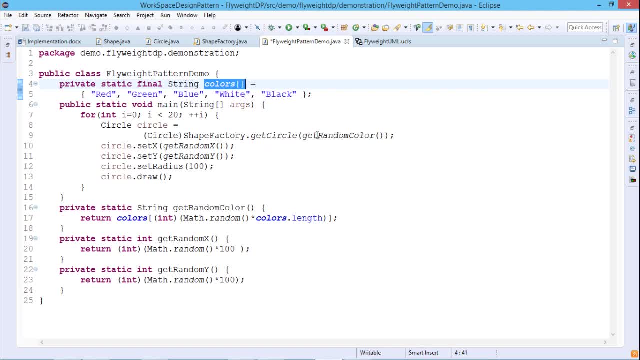 Circle shape factory dot get circle. and here we are having this: get random color. so get random color is use a different function. we have defined that one. so it is using the random method here. so math dot random into colors dot length. so colors dot length is 5 here. so as a 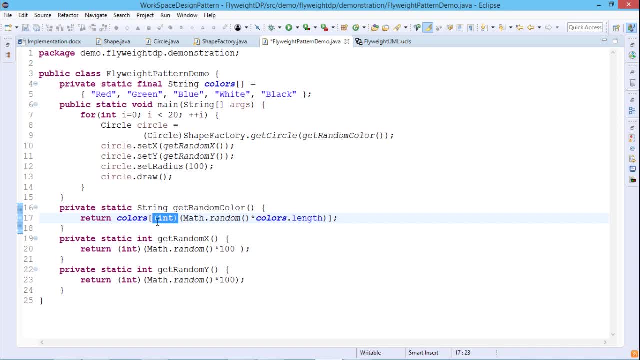 result of that, it will produce the value and we are doing the typecasting to integer so it will produce a value ranging from 0 to 4. so, depending upon the subscript value, the respective color will be retrieved from this colors string array. so that is about get random color. so, depending 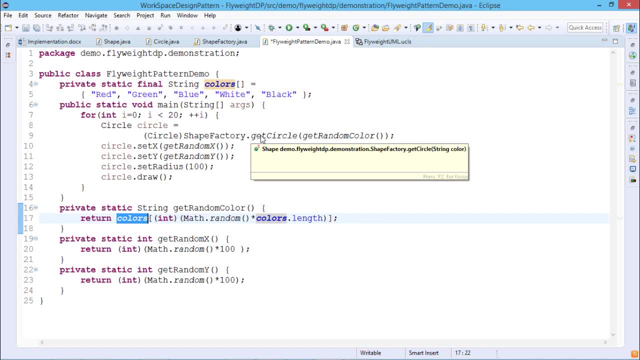 upon the color, the from the hash map object. there is our circle map. we are trying to retrieve the circle object. so that is a circle object we are retrieving. so you know that whenever you are using this, get circle, whenever using this, get circle. so actually this particular method is getting. 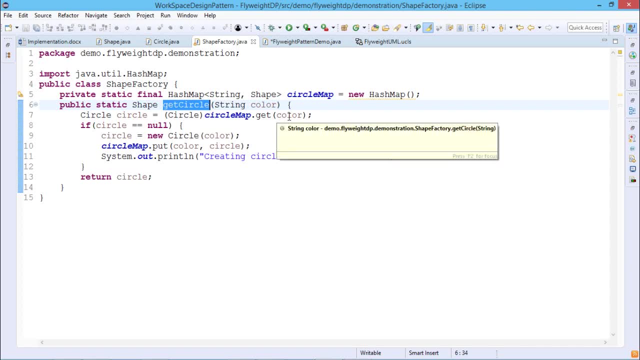 executed. so if the color is the new one, if, if there is no match, then the circle will remain. is equal, is equal to null, then the new circle will be created and that will be put into the circle map. otherwise, the, the, the, the respective circle object, which will be read from this, which will be retrieved from this hash. 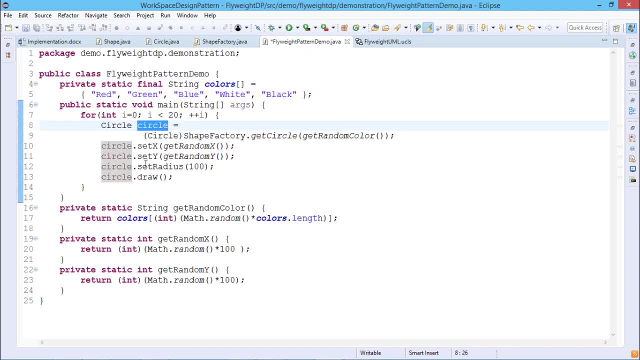 map, circle map will be returned here. so that is the. that is the case, so that this circle will be initialized either using the either newly created circle object or the circle object which will be retrieved from the hash map. so now we are going for this set x, we are going for the set y, we are. 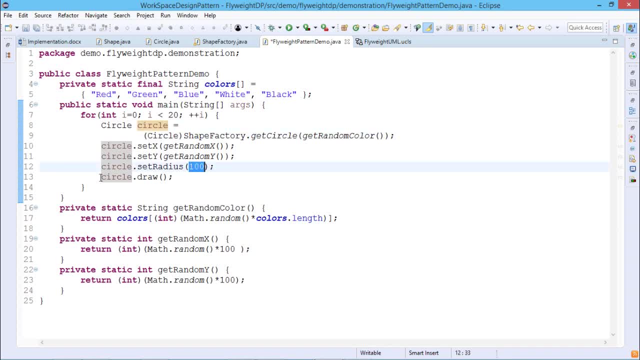 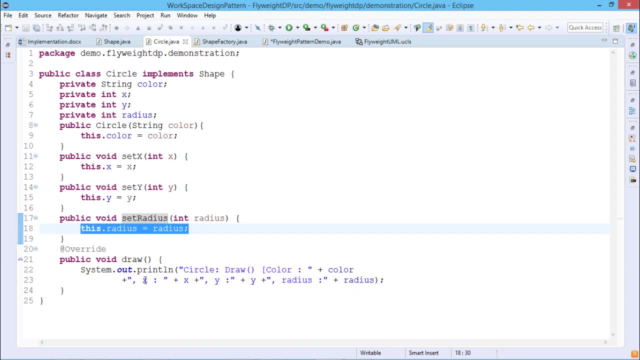 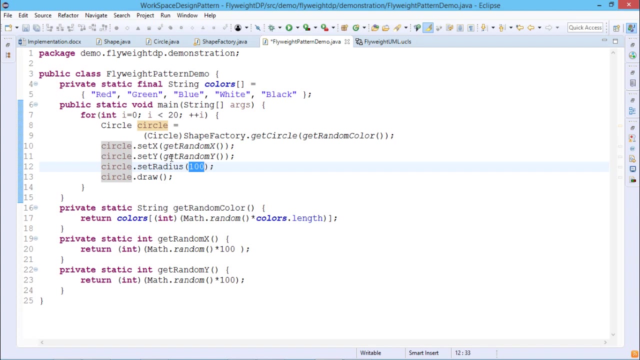 going for the set radius. it is a fixed constant, that is, a 100. and then circle dot draw will be executing this respective method. so there is a, there is a. circle dot draw will print the color, print the x and y coordinates and also print the radius. so that is a, there is a case. so now for this, get random x. for the, get random y. 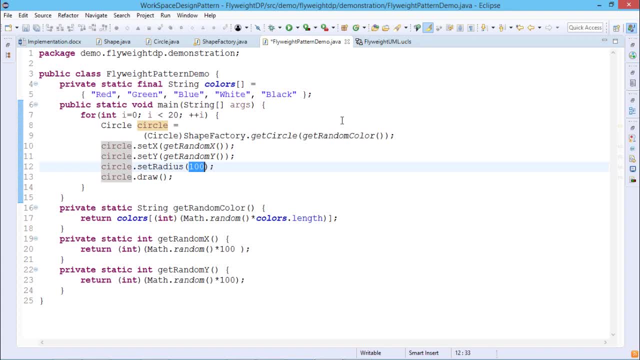 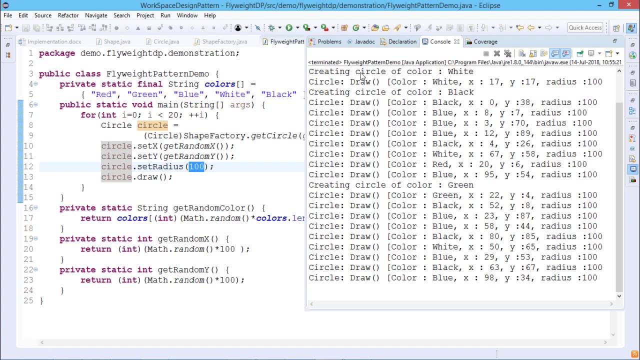 we retain the respective methods here. so now let me go for the execution of the code. you can find that when the white color has appeared for the first time, it is creating the circle of the color white, and then it is putting the respective x- y coordinates and the radius. radius is fixed as 100. 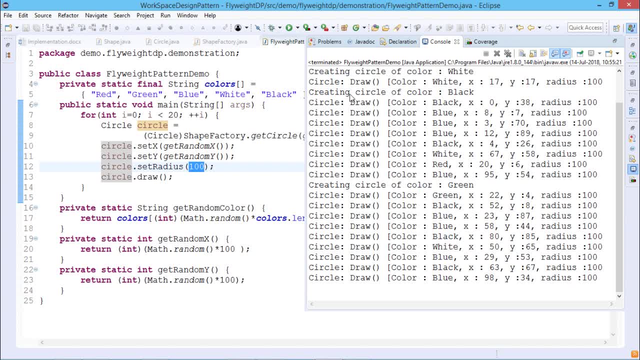 for the black. for the x and y coordinates, the radius is fixed as 100. for the black, for the first time it is creating one object of the circle class and then it is putting the x and y, defining x and y, and put and radius values 100, as again. so now we are going for this blue. i think we should. 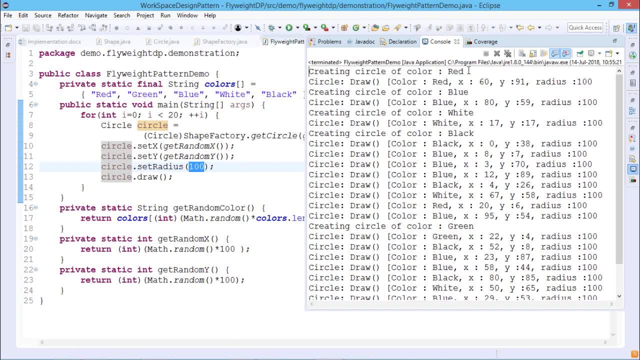 go at the top at first. so for the red, when the red color has occurred for the first time, a new circle object has got created, so x and y and the radius has got printed for the first time. blue, the blue. uh, the new circle object has got created, the x and y and the. 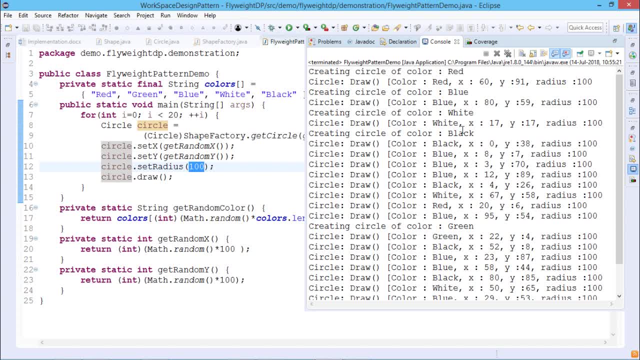 radius is getting printed for the white, for the black. for the first time the new circle objects are getting created. but when we are getting the repetition of the black color, blue color, blue, blue, black, white, red and blue again. so the new objects are not getting created, only the previous object. 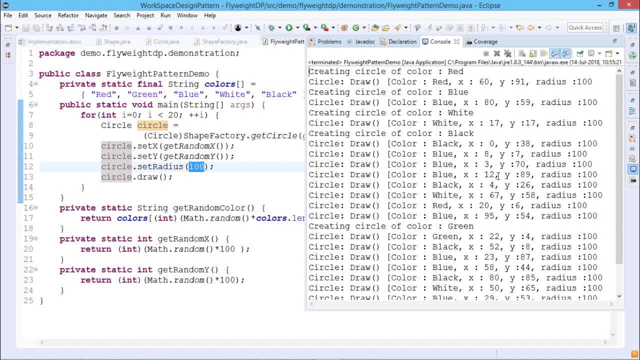 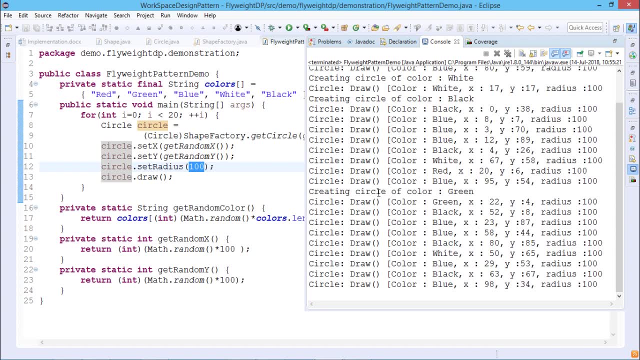 which has been stored in the hash map will be retrieved and new x and y will be assigned and then radius value is permanently 100 here when the green color will come, then for the first time the green color uh, when the green color has been retrieved using the random uh method, that is. 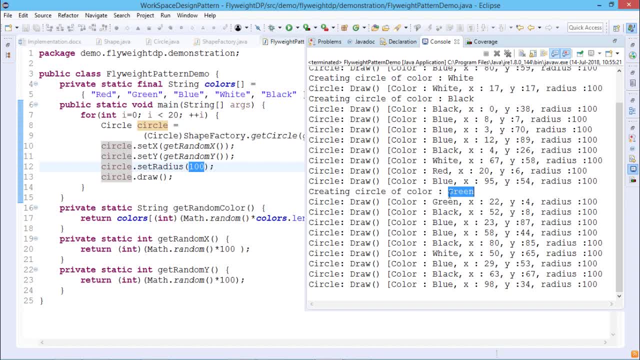 the method we are calling it, and now, when the green color will be will be retrieved from this colors string array, then for the first time, the circle object will be created, and that means we have created objects against the all the five colors, and so there is no scope to create objects. 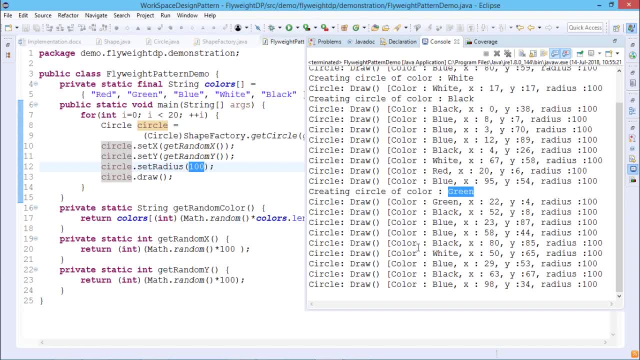 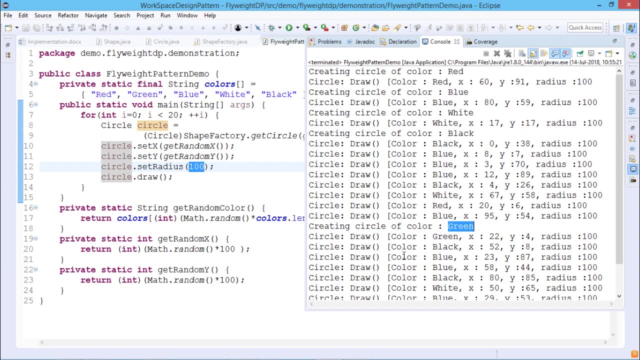 under the circle next. so in this way we can go on creating, go on executing my code and this for loop for 20 number of times where i will be ranging from 0 to 19 here. so this is the respective by outcome. from here we are getting this idea that how this particular flyweight design